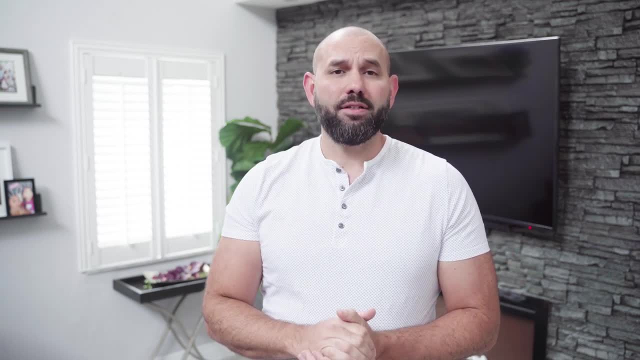 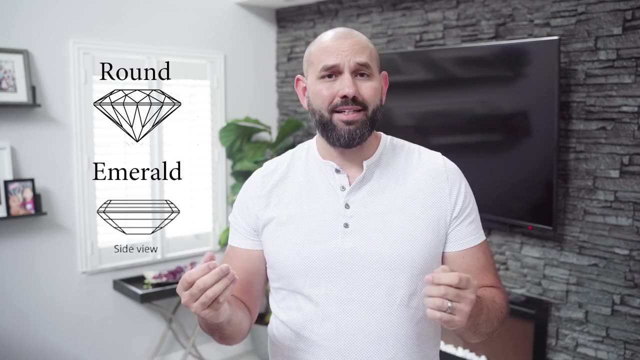 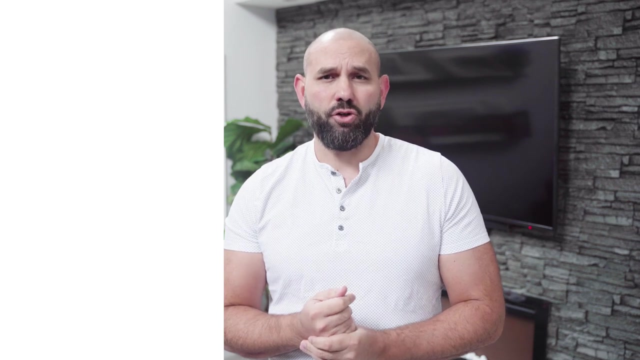 bottom or the side. Round diamond shapes allow for the deepest and smallest surface area on the bottom, Contrast to an emerald which is wide, long and shallow. The bottom point is closer to the top surface, causing the yellow to be more apparent. So quick tips round diamonds. H to J color range is ideal. Princess cut. 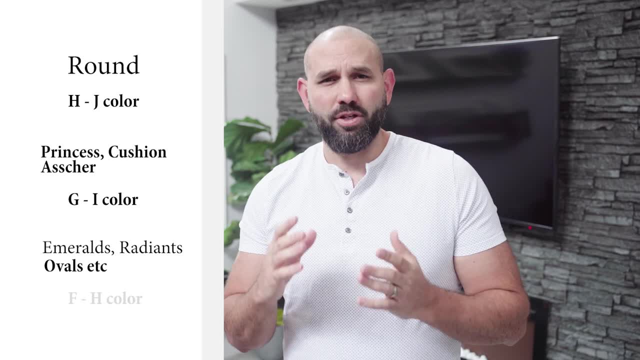 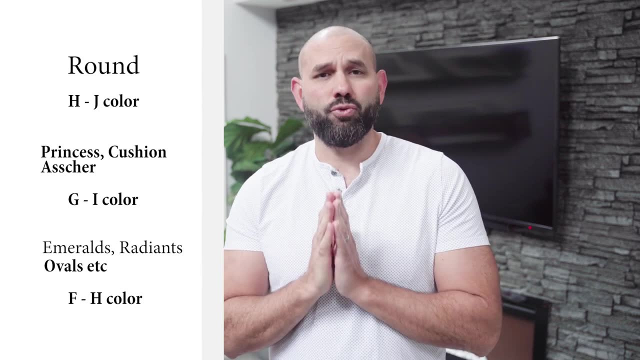 cushion, Asher G to I range, Emerald radiance ovals etc are in the F to H range. Guys, you can go higher if you wish, but the rules of diminishing returns kicks in. It's extremely difficult to see a difference. Money is better spent on a. 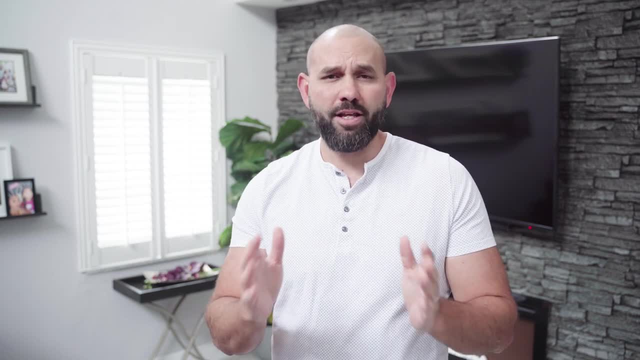 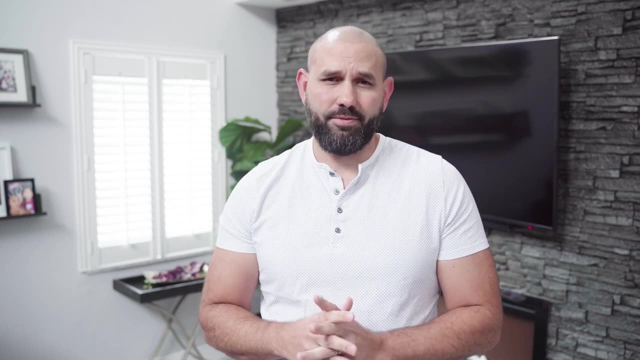 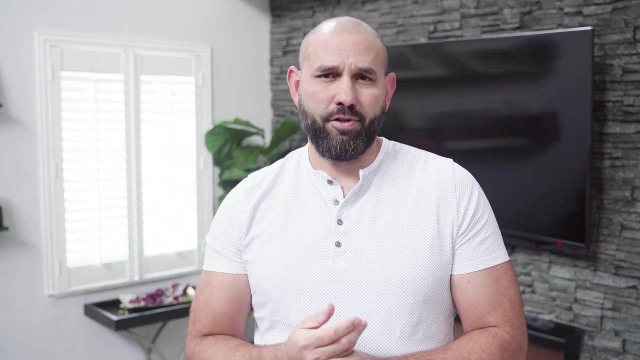 better cut or a larger carat size. Now, if any of your diamond shape choices have diamond fluorescence, it will allow you to get a lower color grade. Which leads me a tip number two: diamond fluorescence, It could be your friend. What is diamond fluorescence? UV light strikes a diamond with fluorescent properties- the stone. 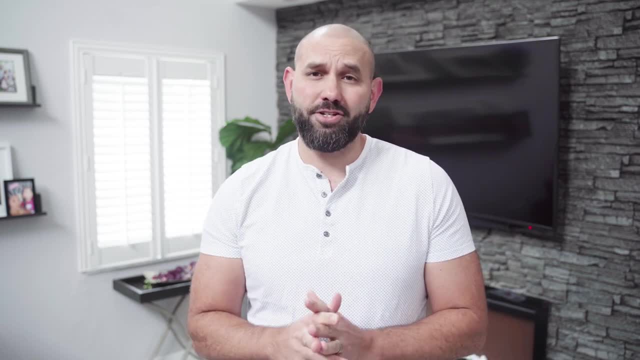 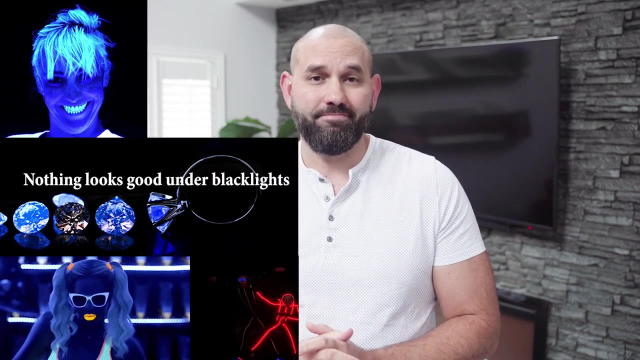 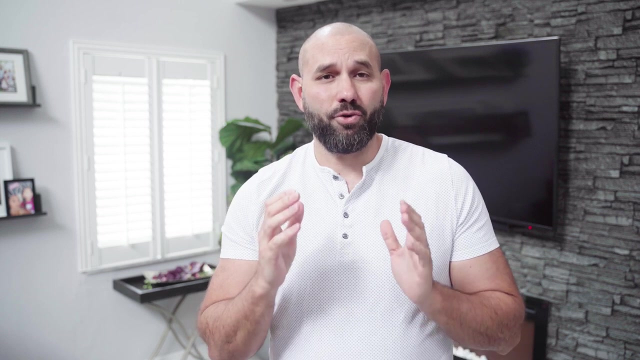 emits a glow. In a quick 9 sign tip explanation, you will go clubbing and you're under a black light. Your diamond will glow like a glow stick. An extremely small percentage of diamonds with strong fluorescence and direct sunlight could make the diamond appear hazy or milky. The diamond has a 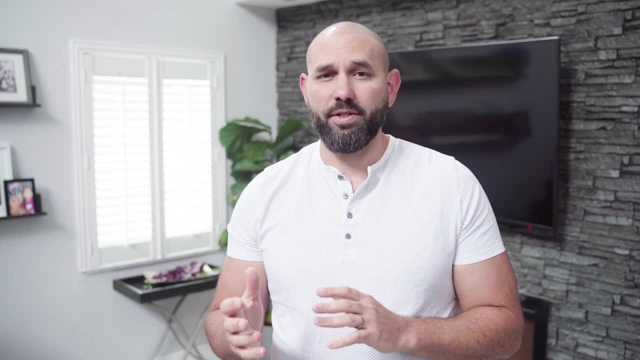 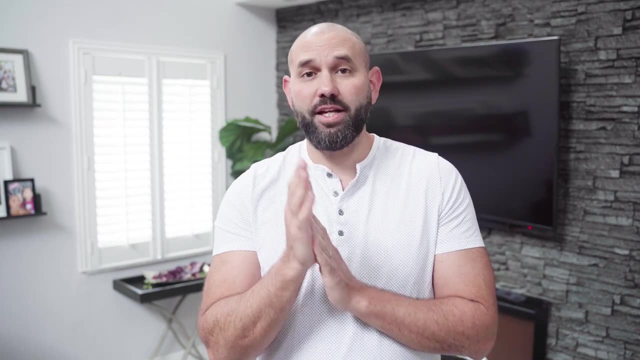 blue property to it that cancels out the yellowing of a diamond, giving it higher color grade. look, So at the end it can help you. For example, you get a J color stone with a strong fluorescence that could cancel out that yellow and looks like you have an H color. 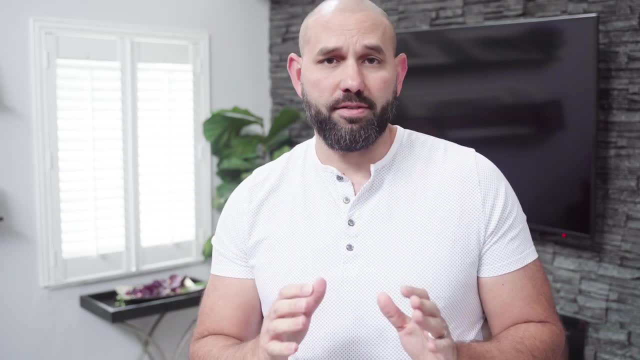 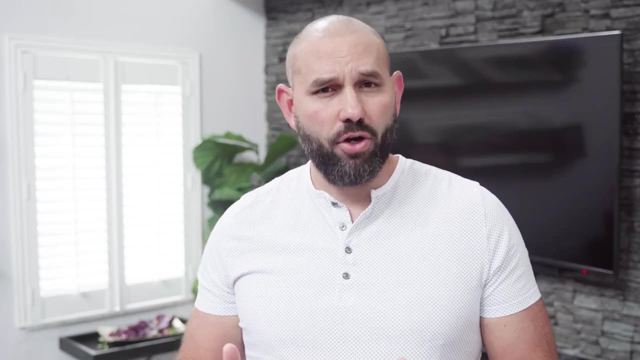 And again, very small percentage of stones are affected by fluorescence. An average person could not make a distinction between stones that have zero fluorescence or strong fluorescence, So, as a buyer, it makes a stone more affordable and gives your lower color grade a bump. Tip 3. The type of gold in your engagement ring will allow you to save money. If it's white gold, you're out of luck, But if you have yellow gold or rose gold, you could easily be in the J to K color range. 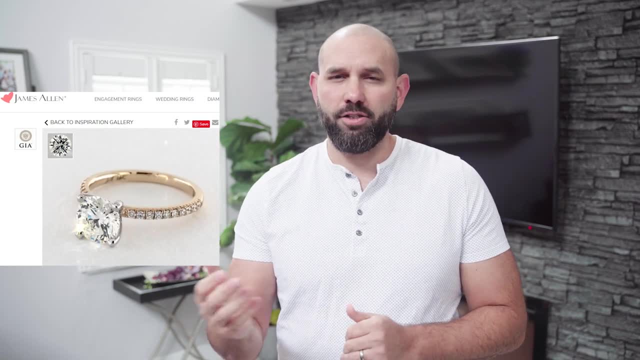 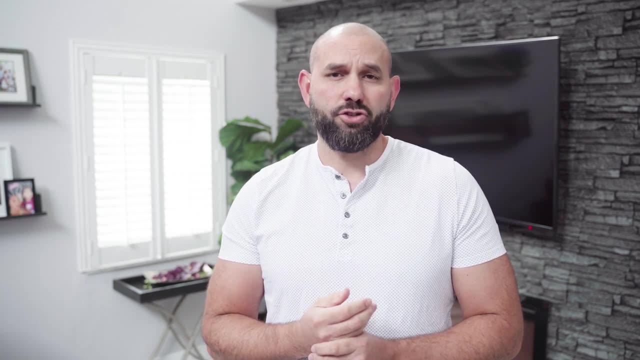 Understand: the light reflects off the gold and affects the color of your diamond. If you have a D color on a yellow gold diamond, it will introduce yellow into the stone, So there's no reason to go crazy on a higher color If this is the case. if you're getting rose or yellow,